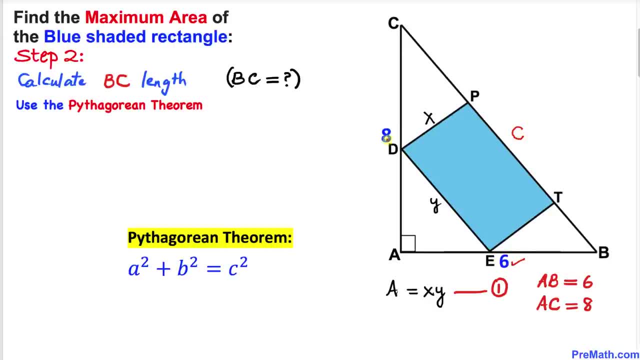 be side c and the other sides are six and eight. so let's go ahead and call this equation as equation number one. and here's our next step. let's go ahead and apply the formula. so this is going to be: six square plus eight square equals to: 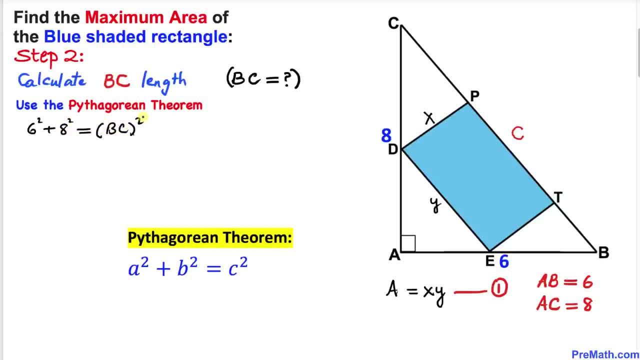 bc square. so therefore, our bc square is going to be equal to 36 plus 64 is going to give us 100. let's go ahead and undo this square by taking the square root on both side. this square and square root is gone and we have a square root on both sides and we have a square root on both sides. 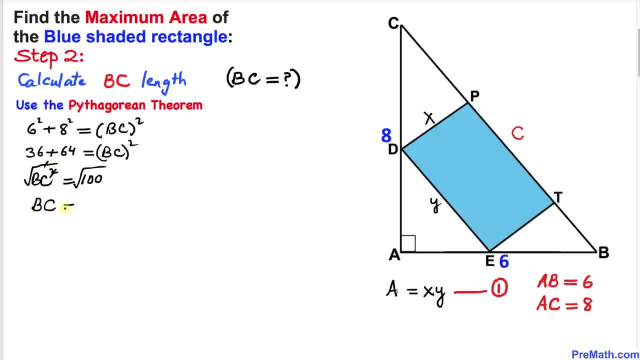 so bc value turns out to be positive 10, and we are going to pick the positive value because we are dealing with the side length. so thus our this side length bc turns out to be 10 units and, by the way, instead of using the pythagorean theorem, we could have used this pythagorean triplets. we could. 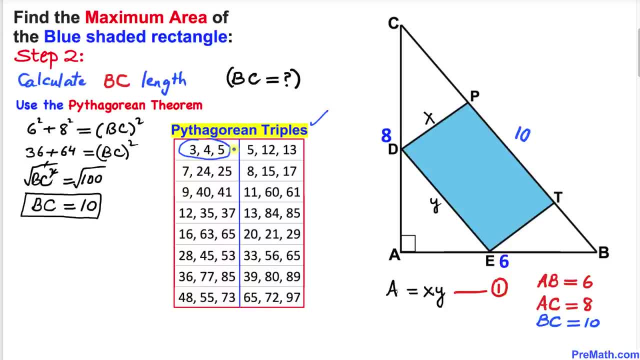 have used this triplets: three, four, five. if we multiply all these triplets, we could have used numbers by two. so three times two is six comma. four times two is eight and five times two is ten, and that's what we have: six, eight and ten. and here's our next step. now we conclude that this: 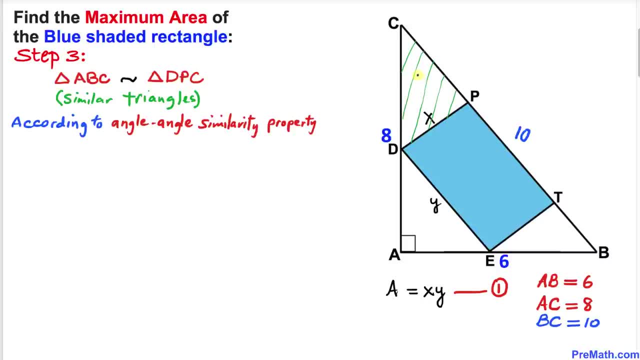 big triangle abc and this smaller triangle dpc are similar triangles according to angle angle similarity property, because this angle is 90 degrees and this angle is 90 degrees as well, and they share this same angle c. and now, before we proceed any further, let me go ahead and call this side cd as length z. 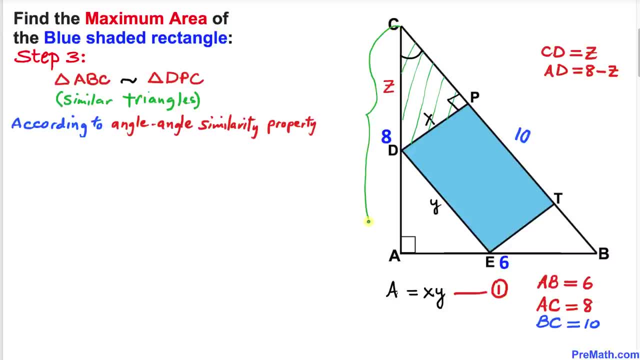 and we know that this whole length ac is eight units. so therefore this side length ad is going to be eight minus z, and then we can see that we are going to have proportion. that means we are going to equate these ratios. we are going to write down z divided by x. 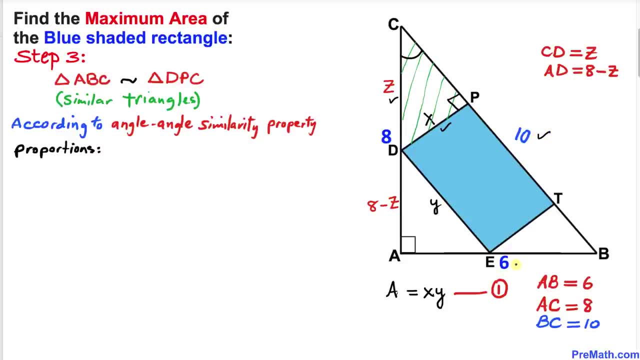 equal to this 10 divided by this six. let me go ahead and write down this one. so i'm going to write down: z divided by x equals to 10 divided by six. now let's go ahead and multiply both side by x to isolate z. so this: 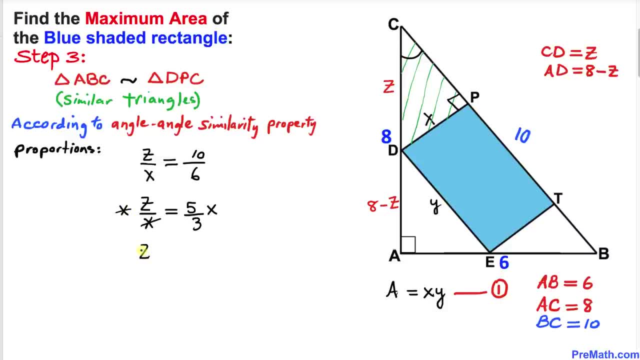 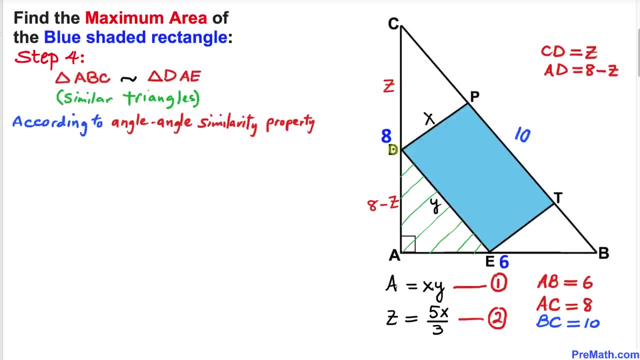 x and x cancels out, so that means z turns out to be equal to five x over three. now let me go ahead and call this as equation number two, and here's our next step. we can also see that this big angle, abc, is also similar to this other triangle, dae, according to angle angle similarity property. 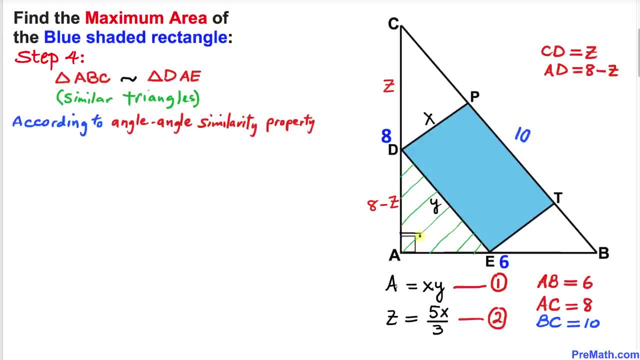 because they share this 90 degree angle and, moreover, this angle and this angle, they are corresponding angles and we can see that they are congruent as well. therefore, we are going to have proportion. that means we are going to equate these ratios. i can write this one y over. 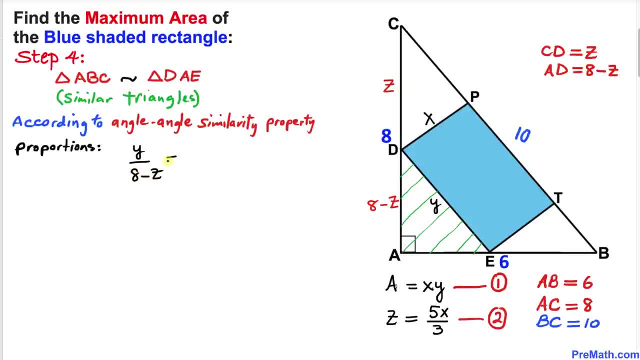 8 minus z equal to 10 divided by 8. and now, on the right hand side, 10 over 8 could be reduced to 5 over 4. let's go ahead and isolate y by just multiplying by 8 minus z on this side. 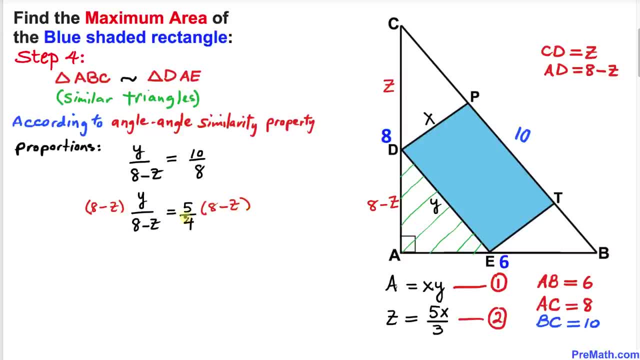 and 8 minus z on this side as well. this is gone. let's go ahead and distribute this one so y could be written as: 5 over 4 times 8 is going to give us 10 minus 5 z over 4. let me go ahead and. 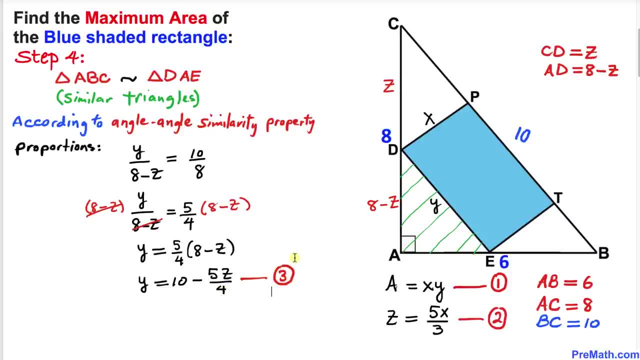 call this equation as equation number three, and here i have put down this equation: three y equals to 10 minus 5 z over 4. and now let's go ahead and substitute z equal to 5 x over 3 from this equation 2 in this equation 3. so wherever we see z, i'm going to replace it by 5 x divided. 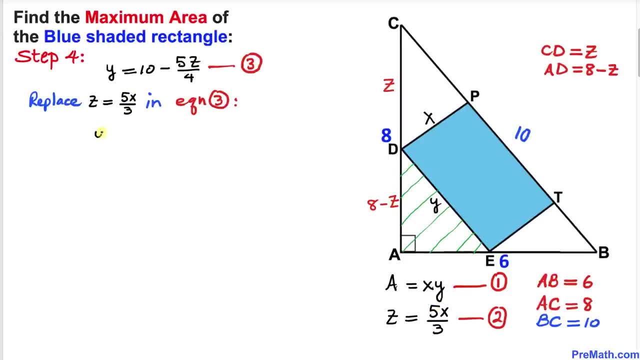 by 3. therefore, our equation 3 is simply is going to become: y equals to 10 minus 5 divided by 3. so let's simplify this thing. so y is going to be equal to 10 minus 25x divided by 12. and let me go. 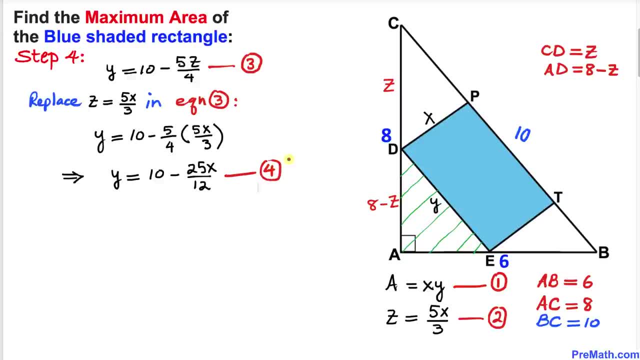 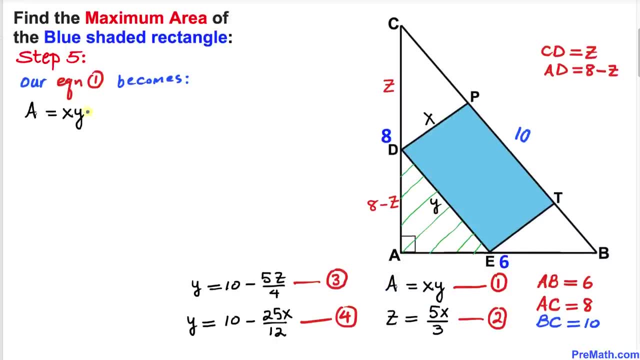 ahead and call this equation 4, and here's our next step. let's focus on this, our equation one, right here. and let's go ahead and call this equation 4. and let's go ahead and call this equation up here and here I have copied it down. let's go ahead and replace this y by this quantity. 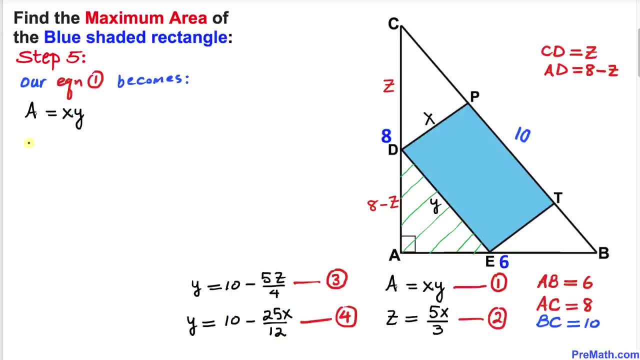 in equation 4. so therefore, this area is going to be equal to x times. I am going to replace this right hand side: 10 minus 25 x divided by 12. and now let's go ahead and distribute this one. so area is going to be 10 x minus 25 x time. x is going to become x square divided by 12. now let 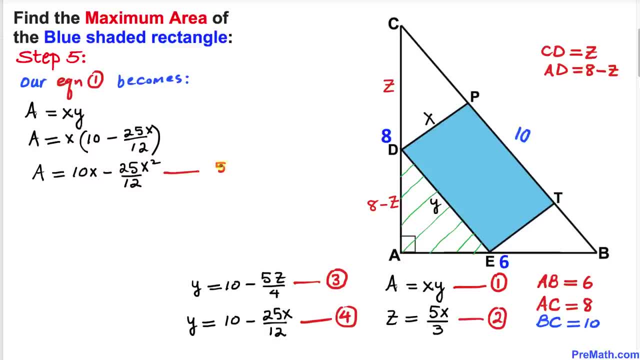 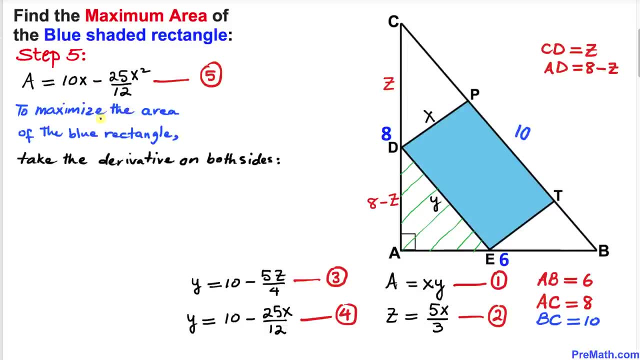 me go ahead and call this equation as equation number 5, and here I have put down our this equation 5, as you can see. and now, since we want to maximize the area of this blue rectangle, so therefore we are going to take the derivative on both side of this equation 5 and just keep in your mind the derivative of a constant a. 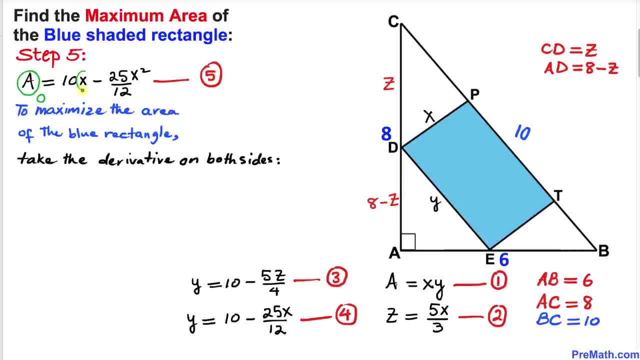 is going to be 0, the derivative of x is going to be 1 and the derivative of x square is going to be simply 2. x- let's go ahead and take the derivative on the left hand side- is going to be 0. equals to 10 times 1 minus 25 divided by 12 times 2. 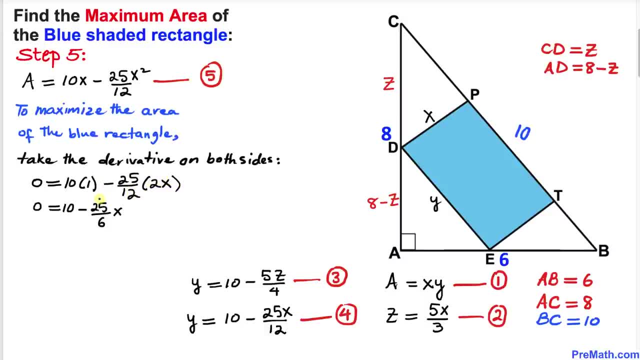 x. and now let's move this negative 25 divided by 6 x on the left hand side. so we are going to have a 25 x divided by 6 equals to 10. now let's go ahead and isolate x by multiplying by its reciprocal 6 over 25 on this side and 6 divided by 25 on this side. so therefore, 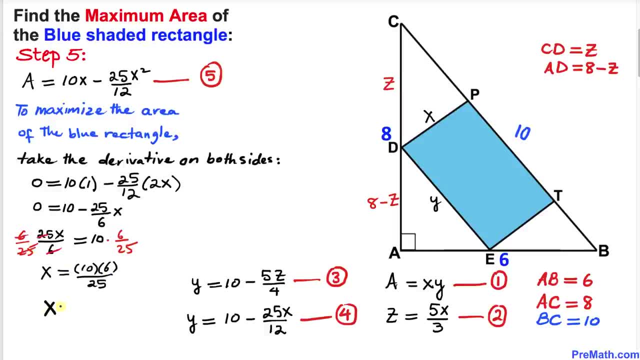 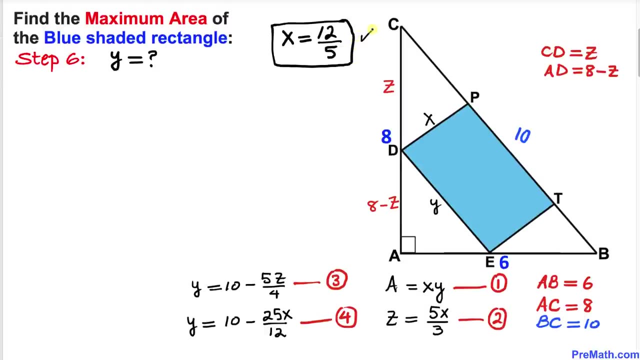 if we simplify on the right hand side, our x value simply turns out to be 12 divided by 5, and this is our x value. and now we can see that our x value turns out to be 12 over 5. and now let's go ahead and calculate the y value. now let's go ahead and substitute this x value, which is 12 over. 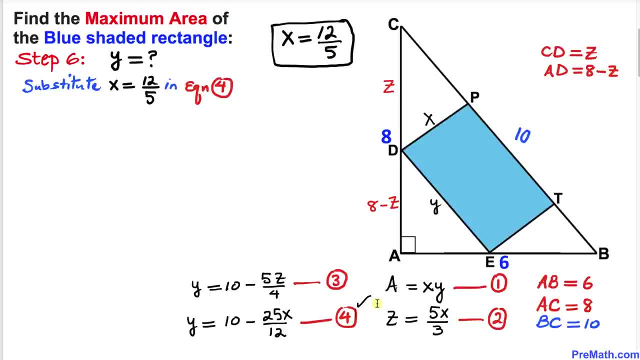 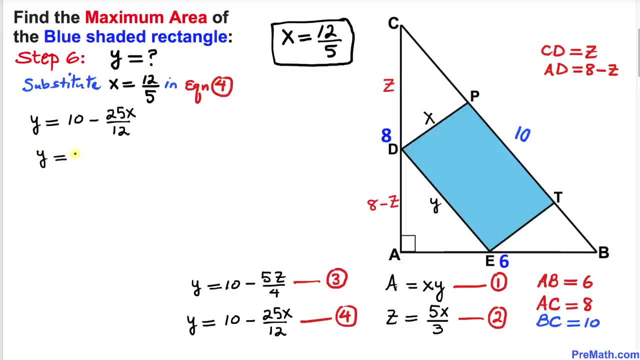 5 in this equation 4. and here's our equation 4. let's go ahead and replace x by 12 over 5, so y equals to 10 minus 25 over 12. and let's go ahead and replace x by 12 divided by 5, so that means y value turns out to: 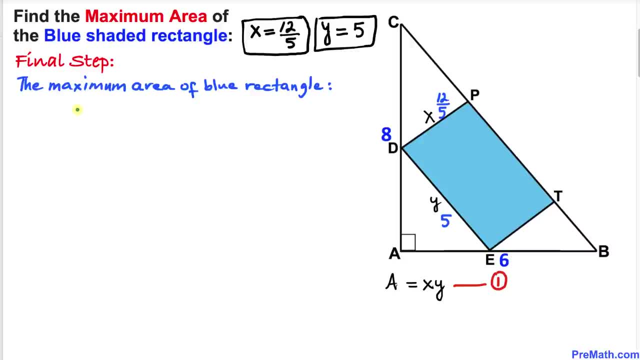 be simply 5. and here's our final step: we are going to calculate the maximum area of this blue rectangle. for that reason we are going to replace these x and y values in this equation 1, and here i have copied down: area equals to x times y equation 1. let's go ahead and replace x and y values over here, so area. 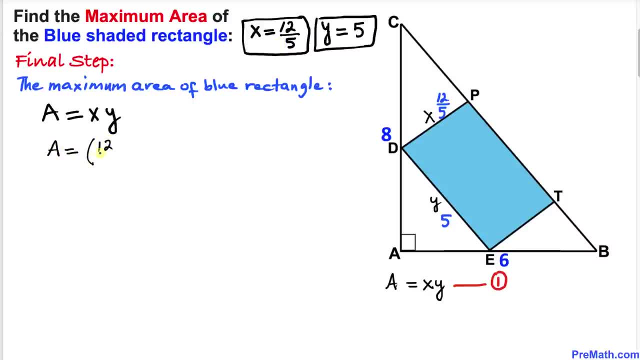 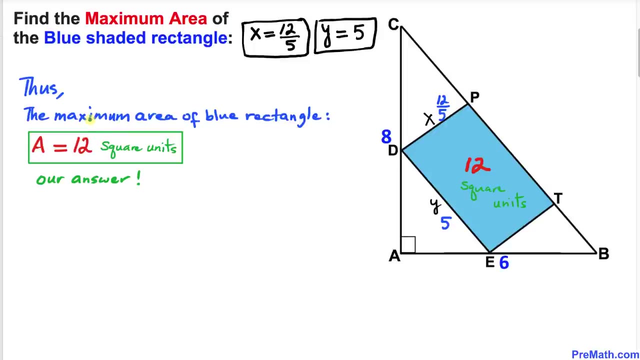 equal to x in our case, is 12 divided by 5 times 5, and here this 5 and 5 is gone, so our area turns out to be 12 square units. So that's the maximum area of this blue rectangle turns out to be 12 square units. 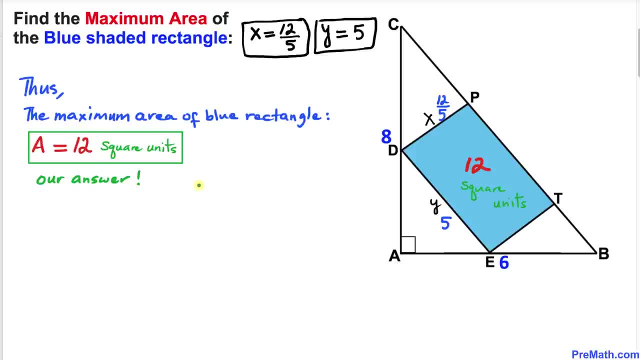 And that's our final answer. Thanks for watching and please don't forget to subscribe to my channel for more exciting videos. Bye.